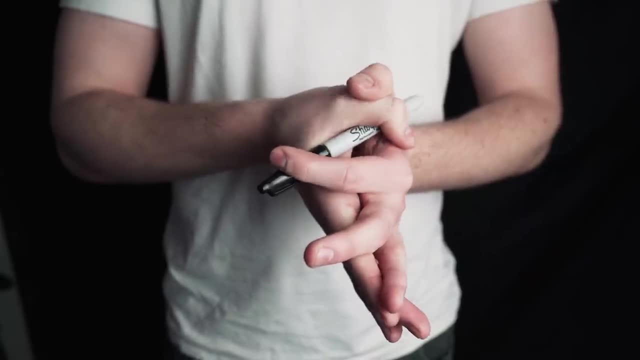 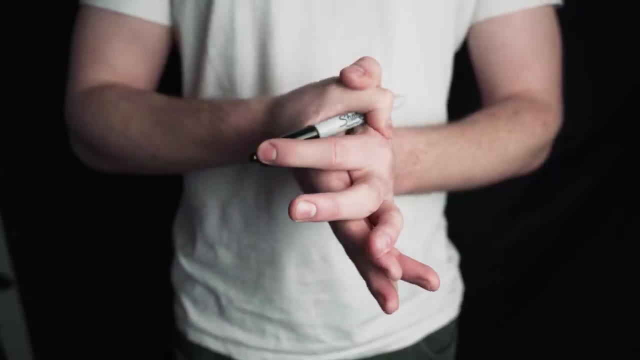 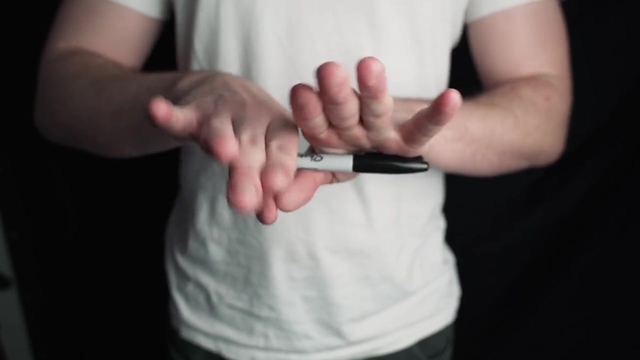 pull the pen towards you. So this finger is pulling the pen this way and this finger is pulling the pen towards you. You then just keep this motion going round, round, round, round round and the pen will go under. Then you just keep practicing this over and over again and eventually you'll be able to do this. 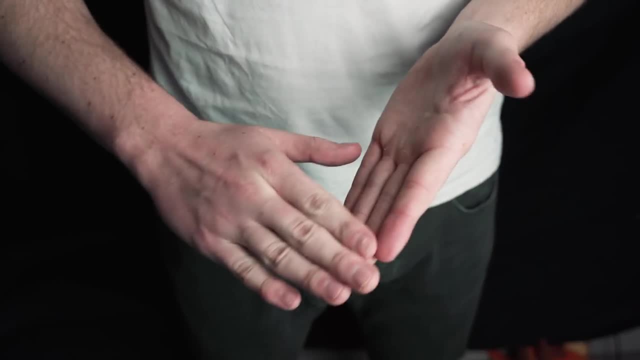 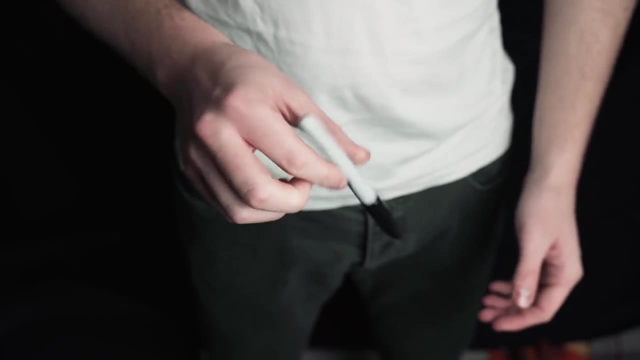 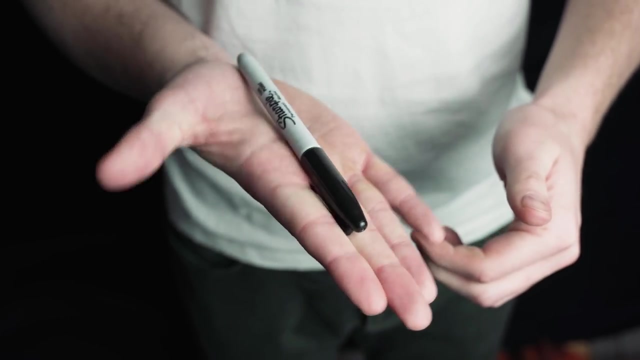 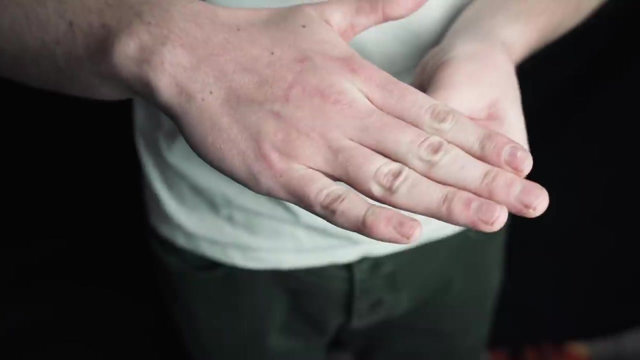 quickly. The magician brushes his empty hands like this and then produces a pen. How is this possible? Clip the pen between your first finger and middle finger with the pen clip. Now just brush both sides of your other hand and then pull the pen out to produce it. 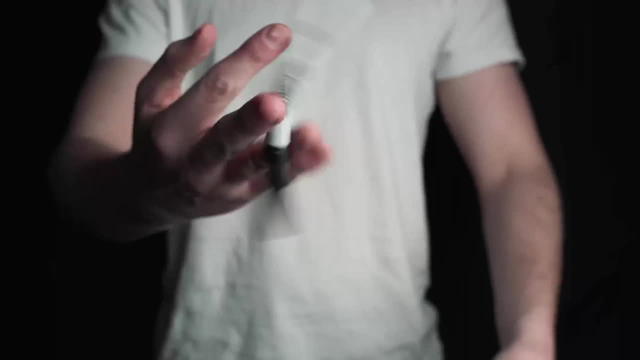 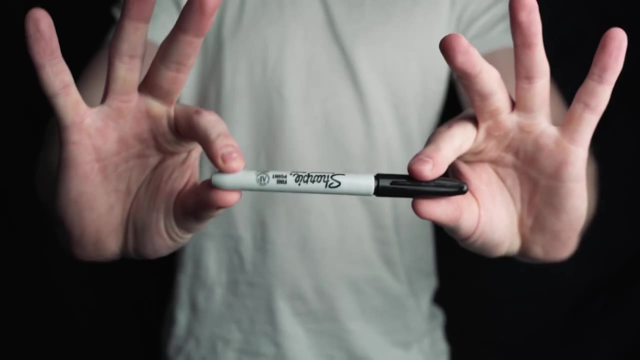 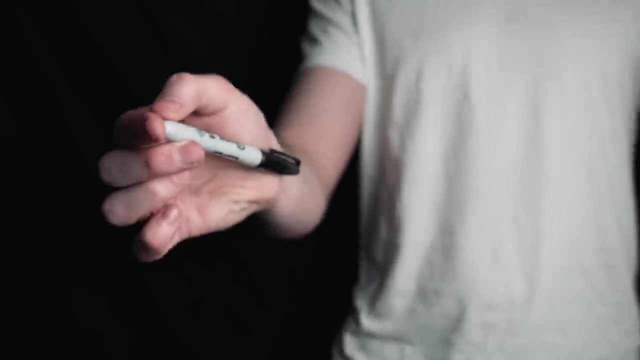 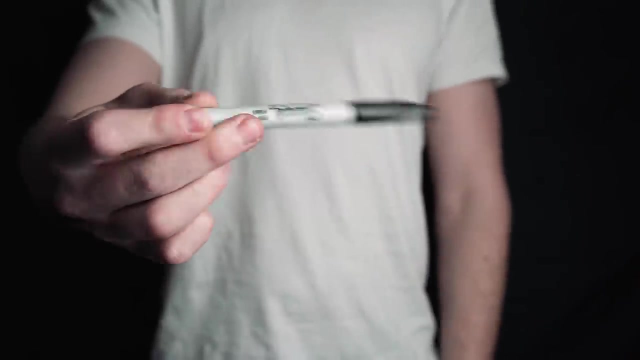 Imagine being able to cleanly show a pen and then vanish it and then make it reappear. Hold the pen between your first finger, middle finger and thumb. Extend your middle finger slightly and then pull the pen back. Keep doing this until it's smooth. Use your thumb to push the pen back out. 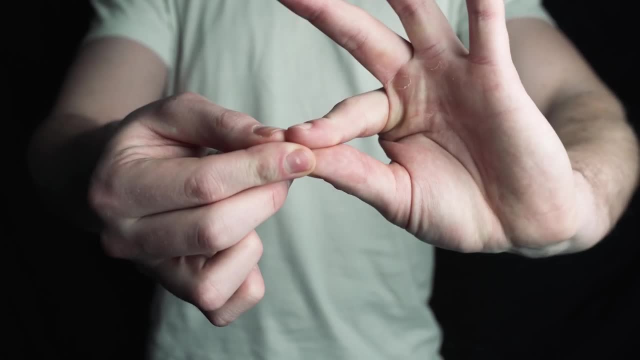 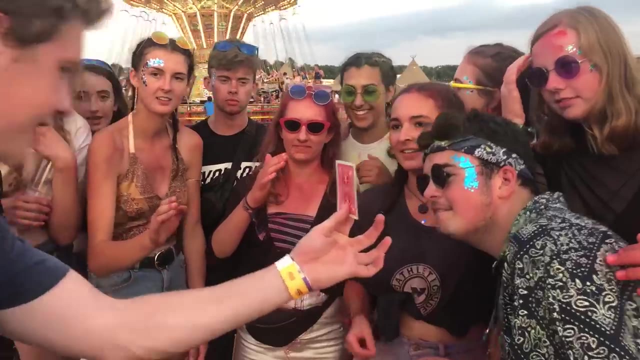 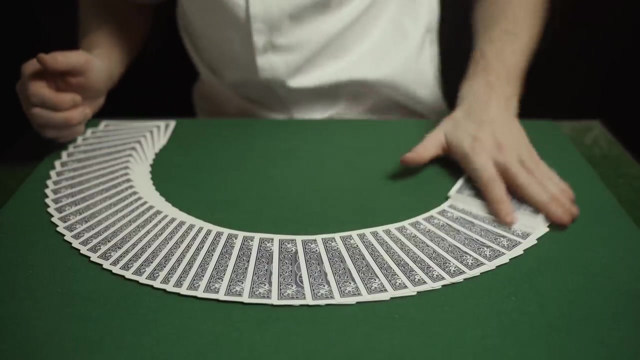 Then simply do this move under the cover of your other hand, and the pen will appear to vanish. If you're interested in learning amazing card tricks that are just too good to reveal on YouTube, then please check out my online card course, Card Magic Pro. It will teach you everything you need to know about card. 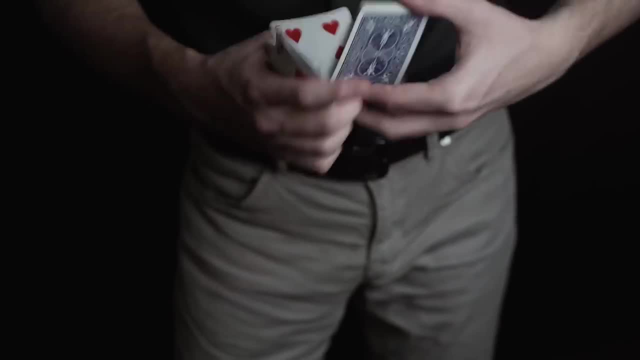 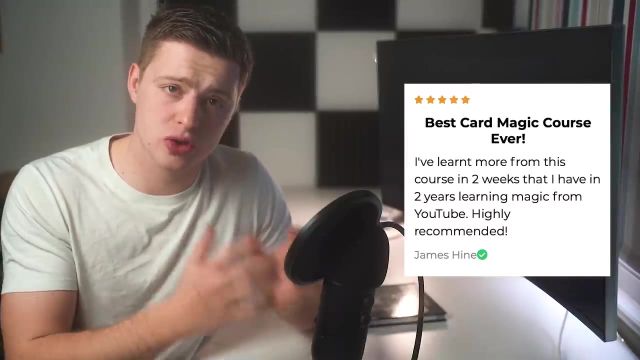 tricks, starting from the very basics all the way up to more advanced tricks and slights. So several thousand people have already joined the course and they've said how they learned more from this course in just two weeks, Then in two years of learning magic on YouTube. I teach you what I think the 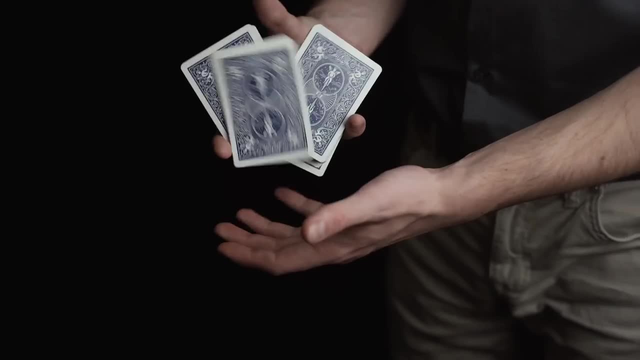 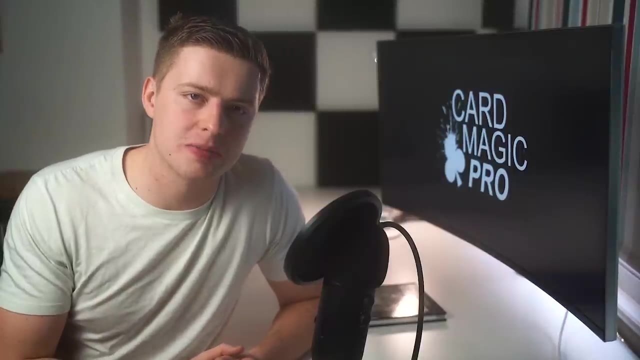 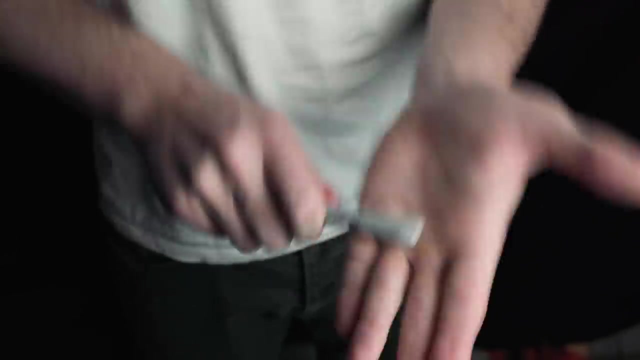 best card tricks ever created, and these are tricks that you can literally take with you to any social situation and amaze whoever you're with. So if you're interested, please click the first link in the description to check it out. The magician taps the coin with the pen and the coin vanishes. How is this possible? 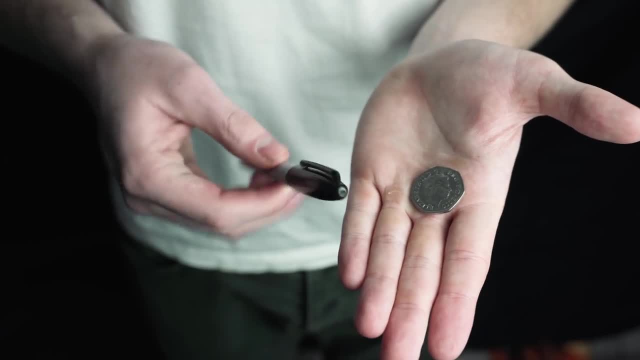 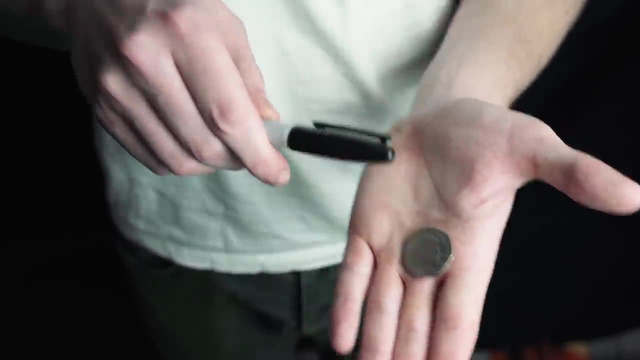 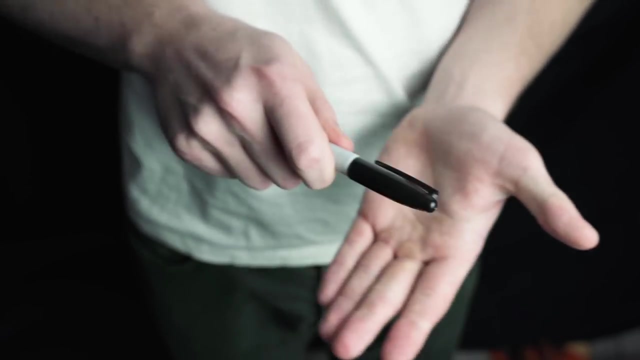 Place the coin into your palm and then the pen in your other hand. Make sure your fingers that are holding the pen are loose like this: Now tap the coin three times and on the third tap, toss the coin into your other hand. Practice this over and over again and 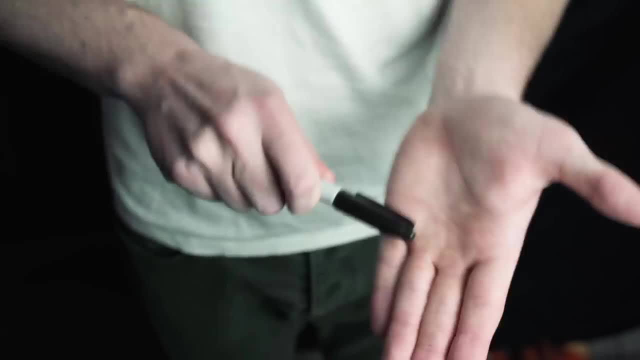 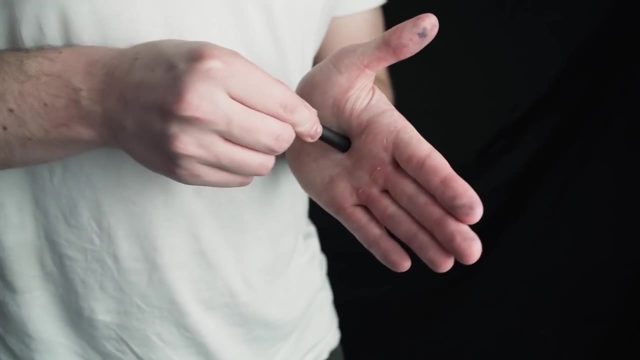 eventually it will look as if the coin is impossibly vanishing. The magician pushes the pen into his hand. He shows both sides of his hand. This is a fun illusion that looks really cool. If you're interested in learning magic on YouTube, then click the link in the description to check it out. 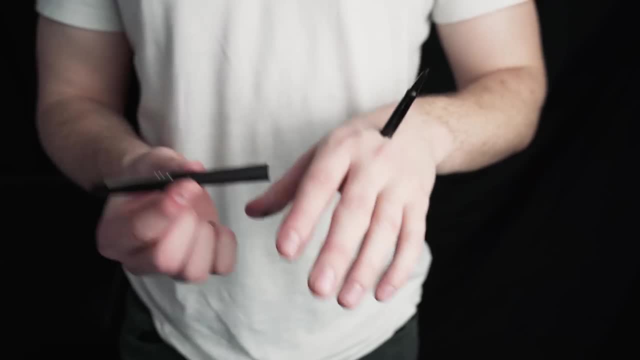 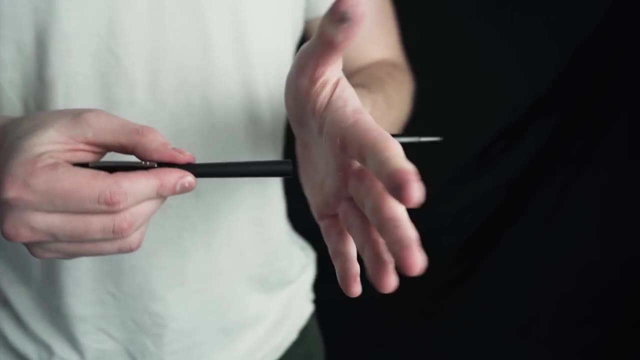 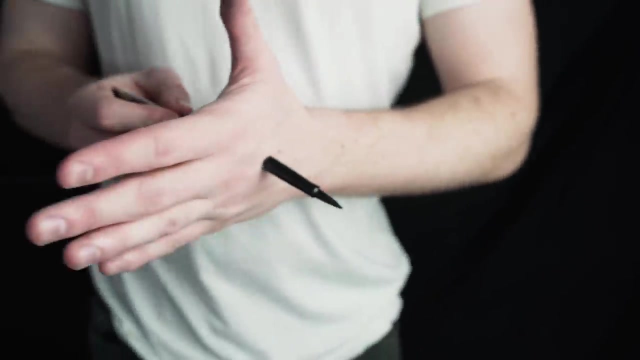 Simply take apart the pen and then stick one part to the back of your hand like this with double-sided tape. Then slide the pen, cap up the pen to create the illusion that it's going into your hand. When you put together, it creates a very convincing illusion If you're looking for really unique and beautiful. 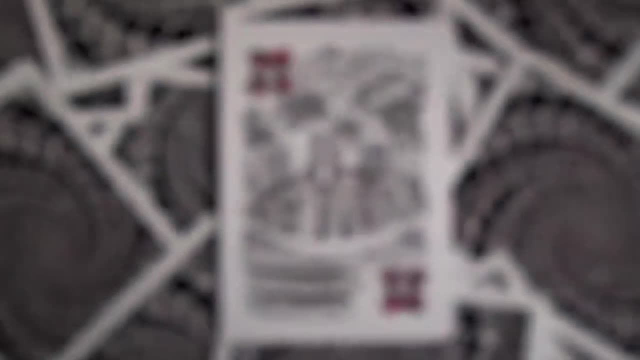 deck of cards to use, then check out the Battle of the Gods deck on Kickstarter. It's one of the best decks I've ever used, with stunning artwork on both the front and the back. If you're interested in learning magic on YouTube, then click the link in the description to check it out. 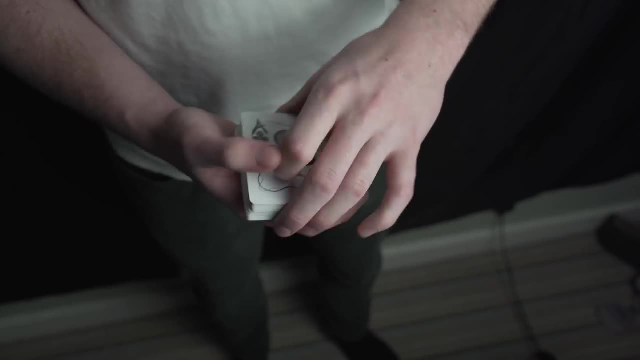 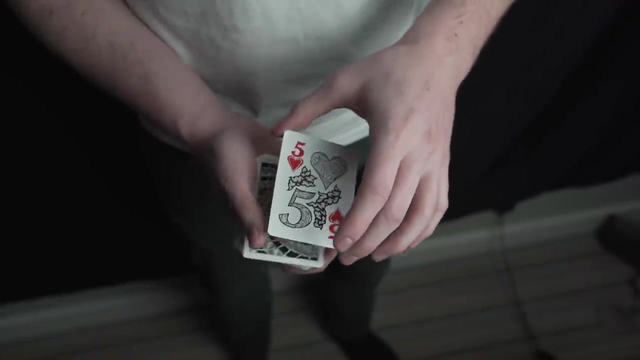 The deck is made out of three different types of cards: The back, the front and back of the cards. They handle really well and they just look amazing. So go and check them out by clicking the link in the description and back them on Kickstarter and get your deck before they all sell out. The magician has a. 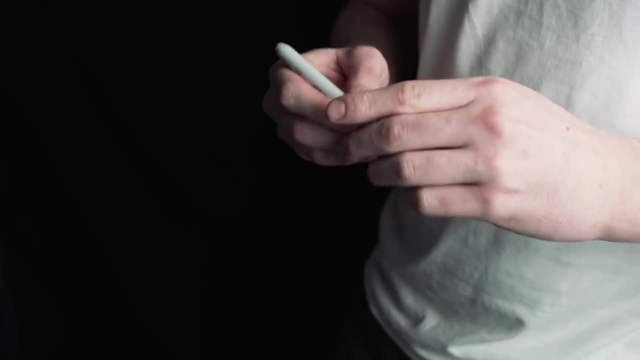 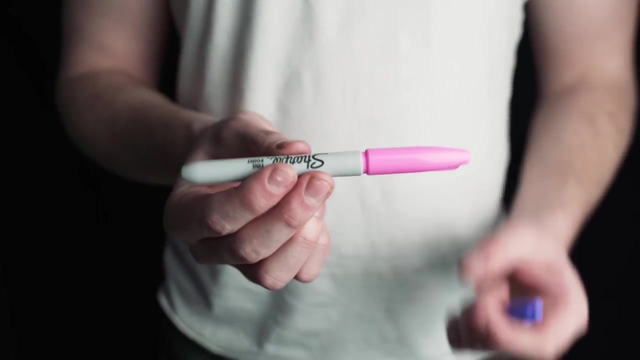 blue pen takes off the cap and then the pen turns pink. This is a very simple effect. Get one sharpie, take off the cap and put it on the other end, then get a different color cap and put it over the next one. This is a very simple effect. Get one Sharpie, take off the cap and put it on the other end, then get a different color cap and put it over the next one. 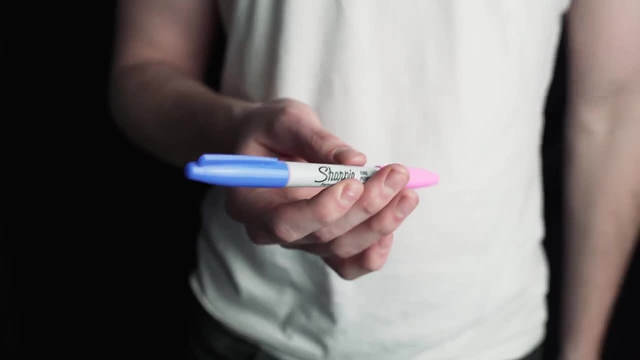 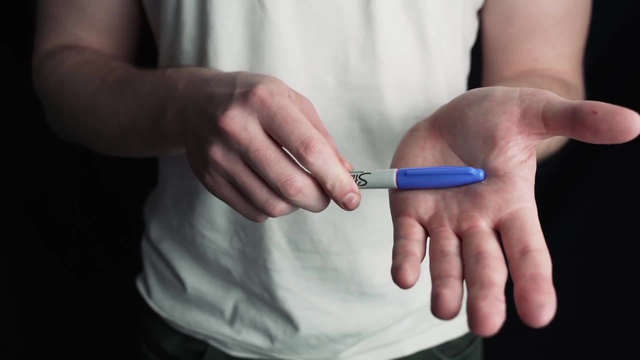 Now what you need to do is begin by displaying this end of the sharpie with the nib under it, hiding the other part in your hand like this: So you display your hand open and then come round and just drop or pull off this part of the 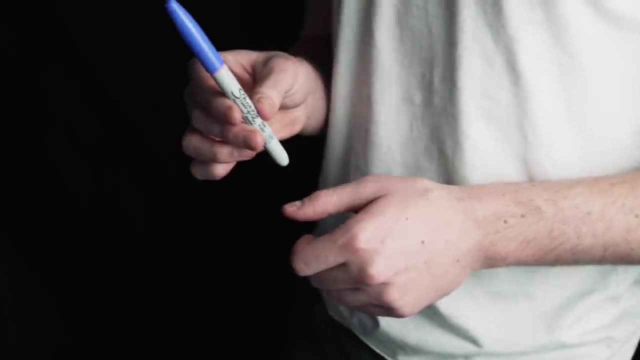 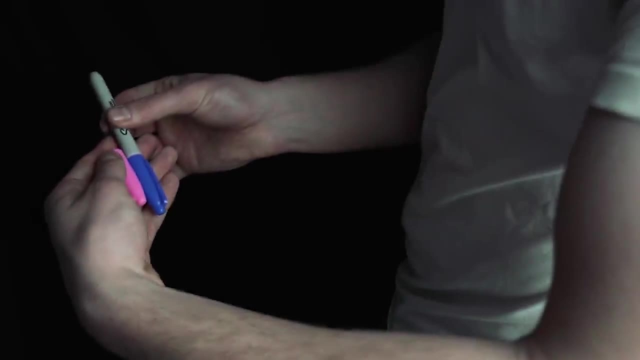 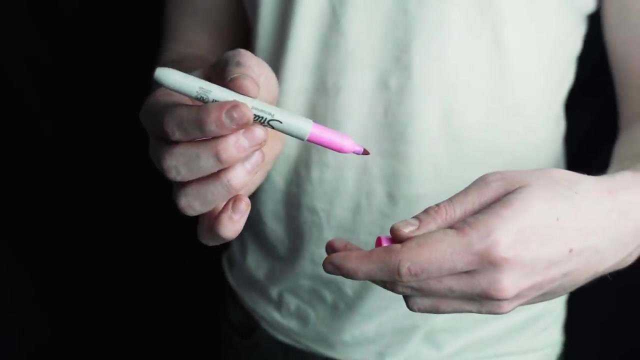 nib into your free hand. So you display your hand clean here and just pull the nib off and pull the cap off like that. So, very simply, this pen becomes behind this other one and then you're going to pull off the cap revealing the different color pen, whilst you also push the other color cap out. and this 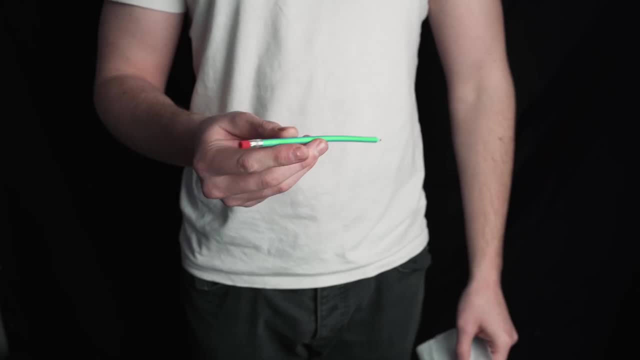 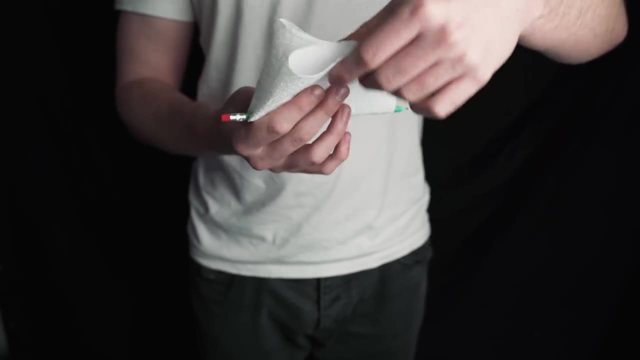 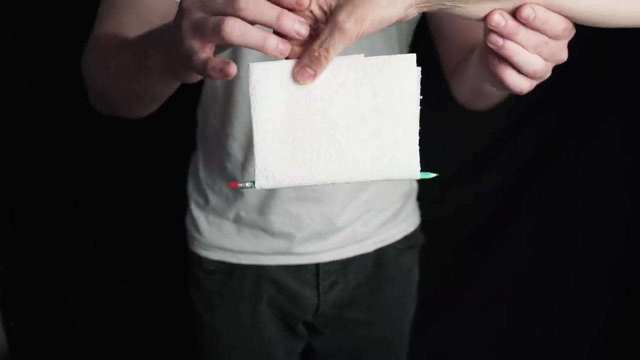 creates the illusion that the pen has just changed color. This is one of the most visual pen tricks I know. The magician takes a pencil and puts it into a folded up paper towel. Everything is clean and fair, The spectator holds everything and then the magician does this: The pencil impossibly vanishes. 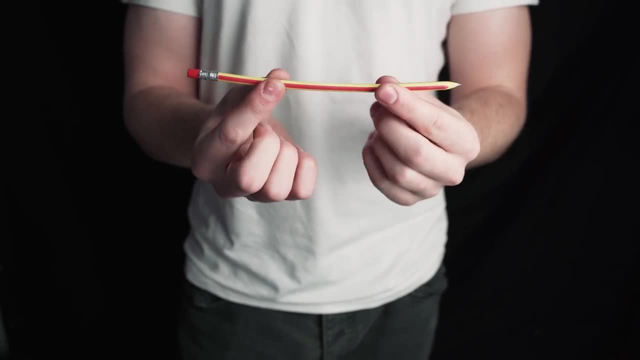 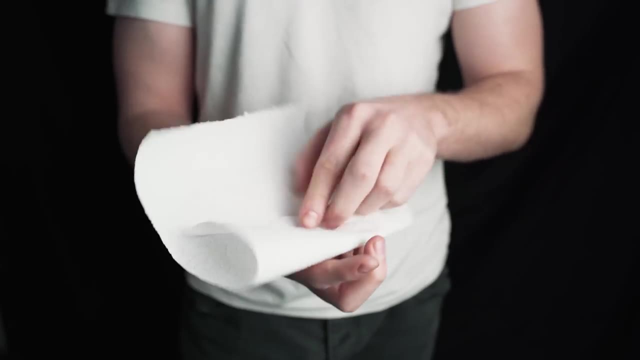 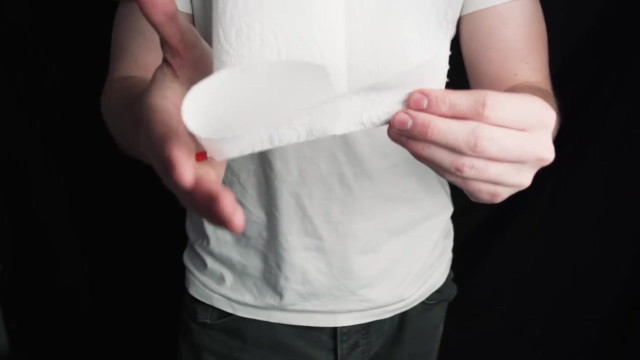 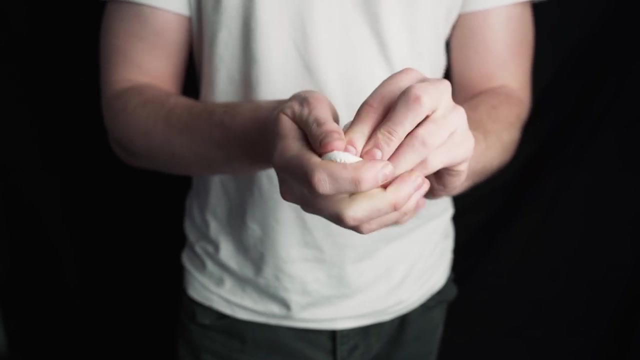 For this trick you need a bendy pencil. You can buy these really cheaply online From here. you simply place the pencil into a paper towel and ask the spectator to hold it. When you crush the pencil, it bends inwards and you can simply put it into a little ball and then put it into your pocket afterwards. 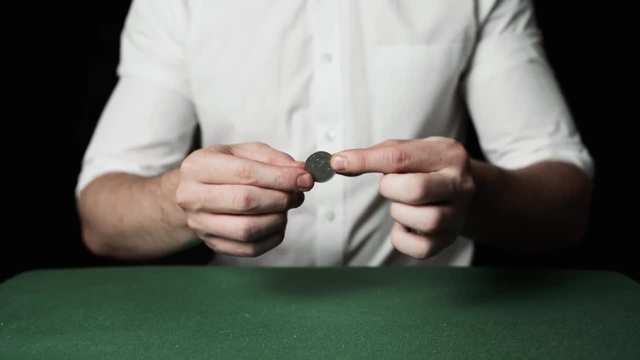 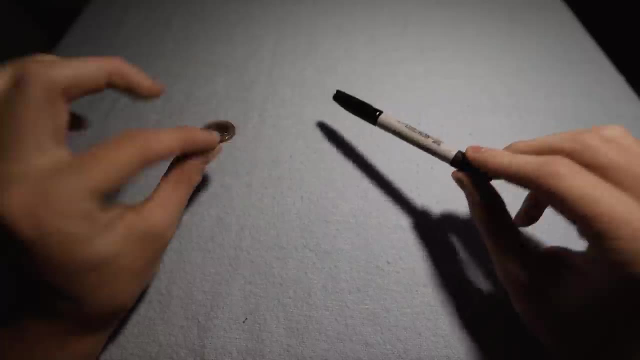 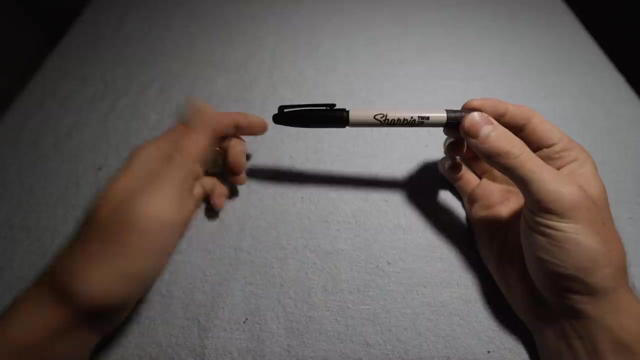 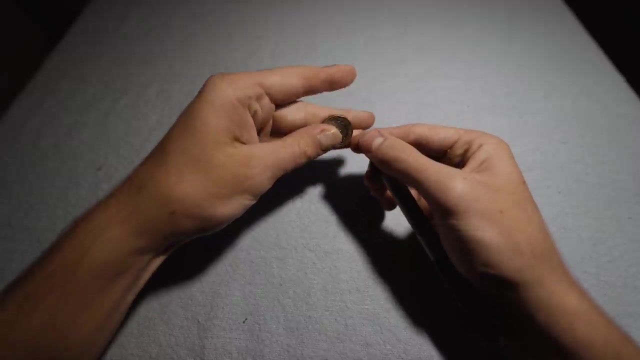 The pen changes its shape. This trick requires a pen and a coin. Practice using your thumb to push the coin upwards in a snappy, sharp motion. Also, practice the flip stick move that I taught earlier. It needs to be very quick for this trick to work. Show the pen and flip it back as you. 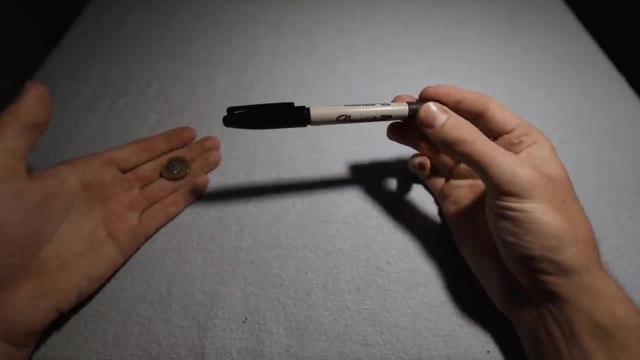 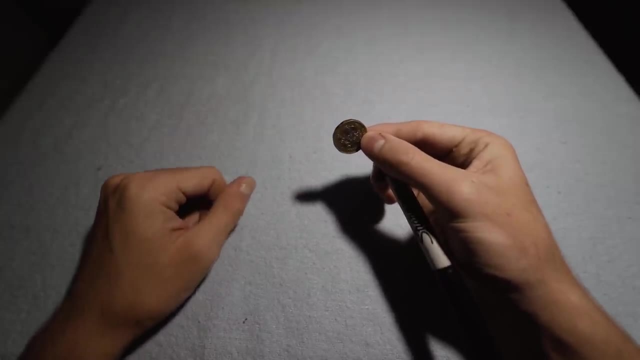 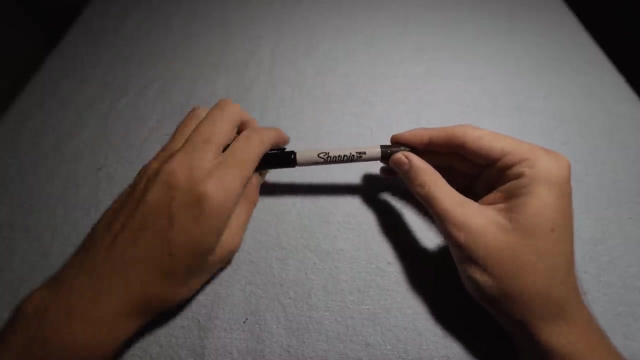 produce the coin. Then practice dropping the coin into your hand, keeping your fingers bent so the spectator doesn't see it when it drops. Produce the concealed pen as you drop the coin. This creates the illusion of a visual transformation. Now simply perform the first move again. 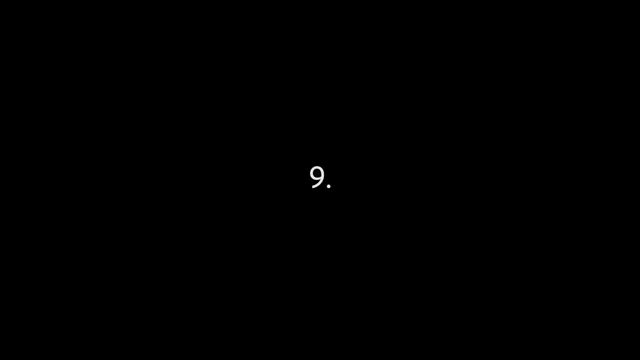 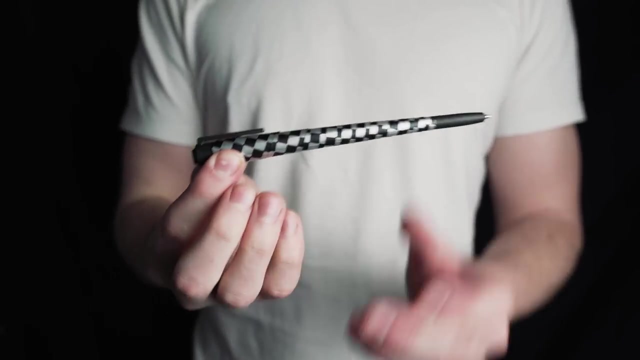 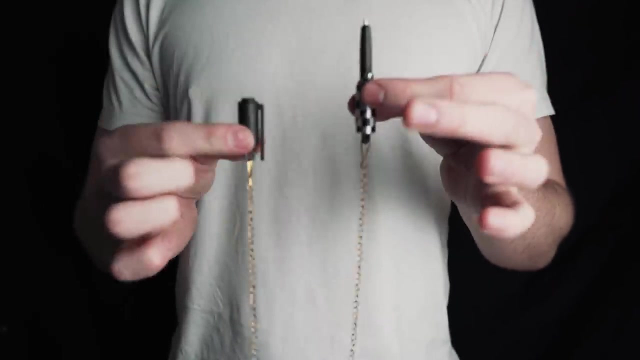 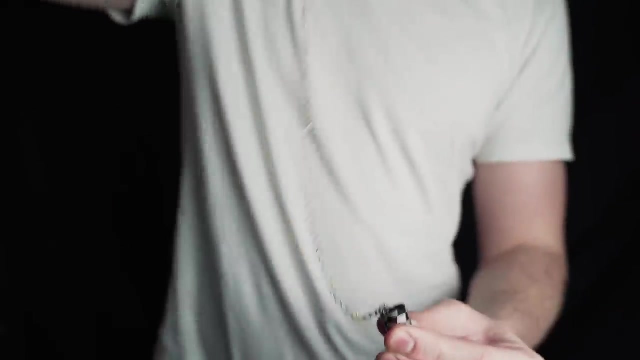 Vanish the pen and produce the coin. The magician has a pen and then it visually transforms into a necklace. This trick uses a gimmicked pen. Inside the pen is a necklace and you'll find the body of the pen is collapsible. You can buy one of these using the link in the description. 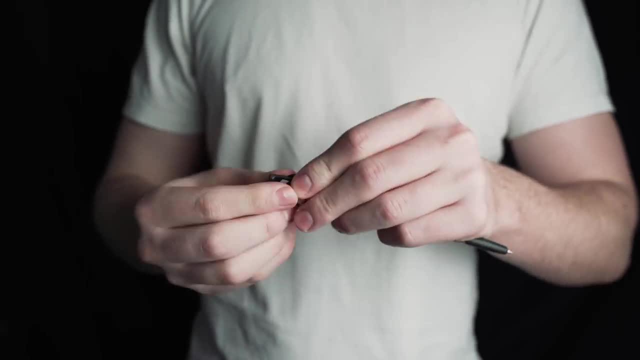 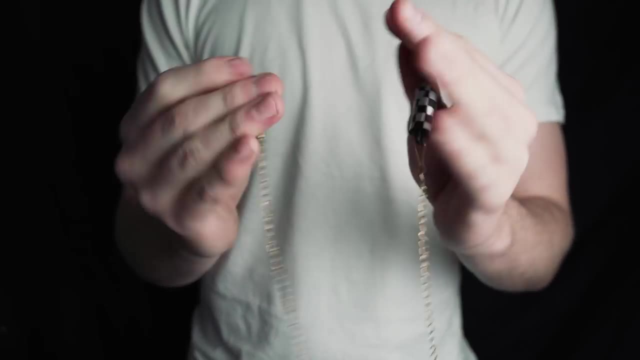 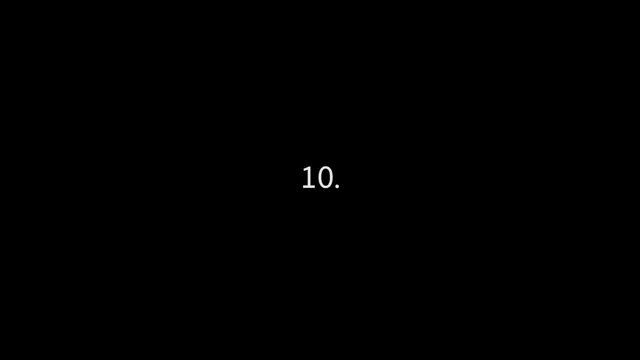 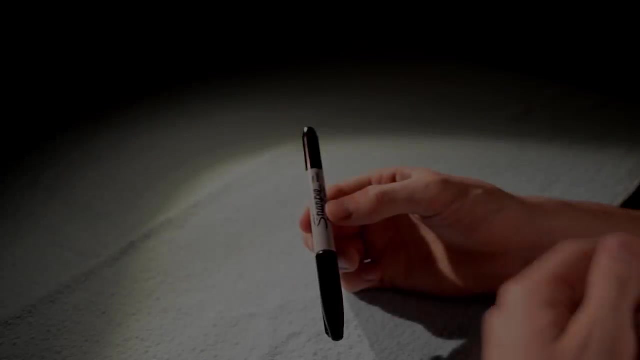 Put the necklace in the body and then hold the pen out like this: When you let go, bring your hands apart like this to reveal the necklace and then put it on. Repeat: The pen lid visually jumps Shade half the top of your pen in black.